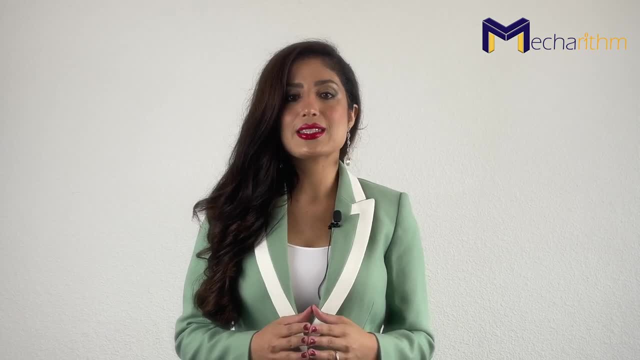 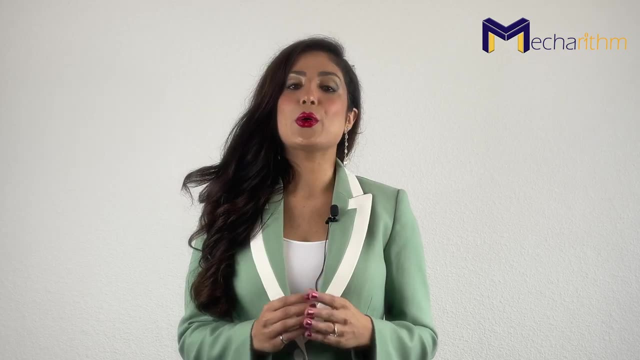 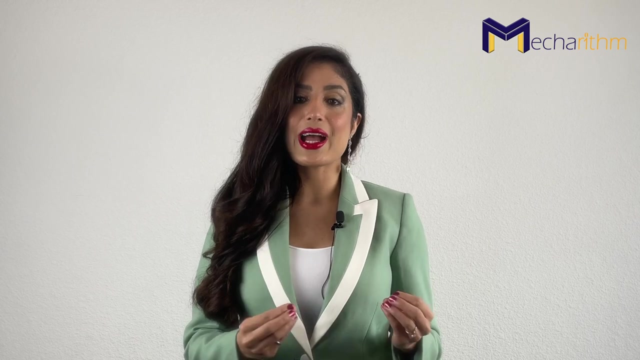 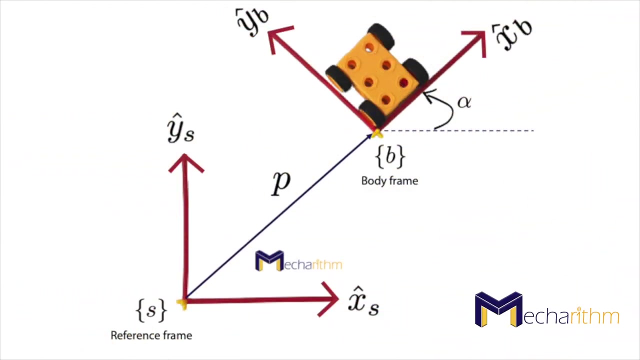 that you watch the configuration and configuration space lesson before proceeding this lesson. You may also want to watch the preliminaries video and also the degrees of freedom video, because the material there can be beneficial to grasp and understand this lesson better. We start this lesson with a planar example to see what we mean with the definition of. 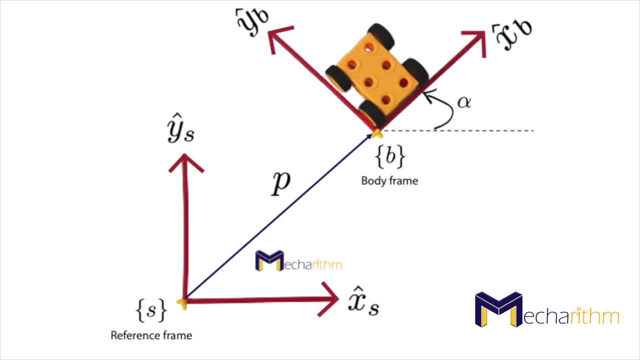 to express the configuration of a robot, Suppose a toy car with its motion confined to the plane, and two coordinate frames, S and V, with their corresponding unit axes. Note that a hat notation shows a unit. vector V is called a body frame, since it's a fixed frame attached instantaneously to the moving body. 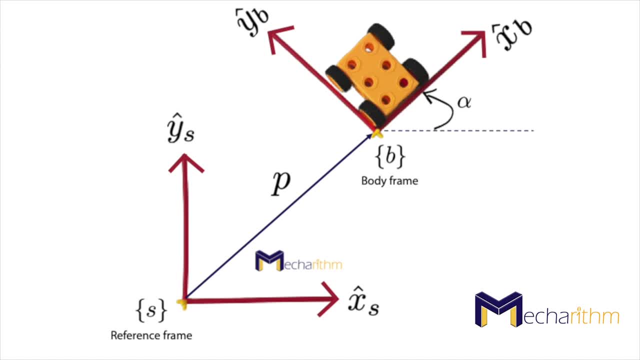 Therefore, to find the configuration of the toy car, you should express the position and orientation of the body's fixed frame coordinates in the base frame coordinates. One way to represent the orientation of the body coordinates in terms of the base coordinates is using a rotation matrix. 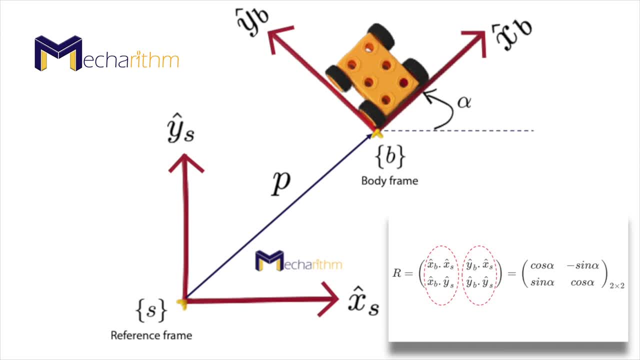 The columns of this matrix are the coordinate axes of the B-frame expressed in the coordinate axes of the S-frame. The dot represents the dot product between the coordinate axes and, since they are unit vectors, the dot product represents the cosine of the angle between the two vectors. 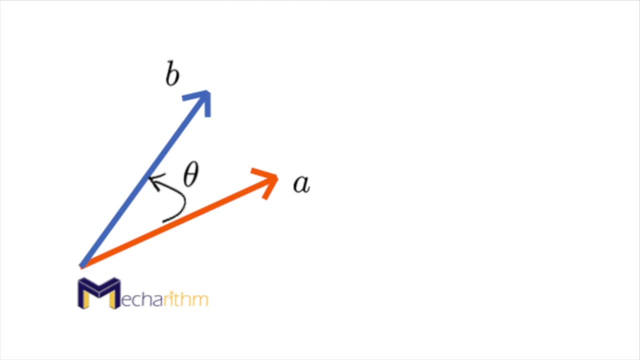 As a reminder, recall that if A and B are two vectors with known lengths and angles between them, then the dot product of two vectors is the multiplication of the lengths of the two vectors and cosine of the angle between the two vectors, In other words the dot product. 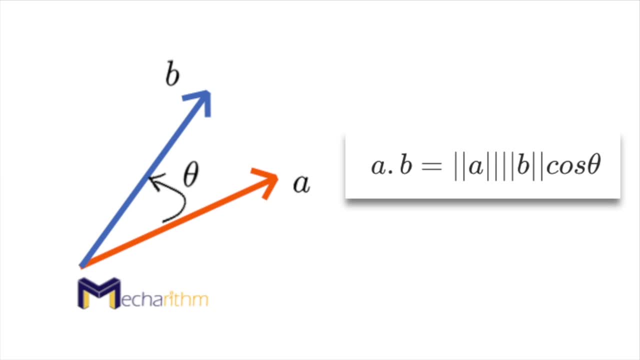 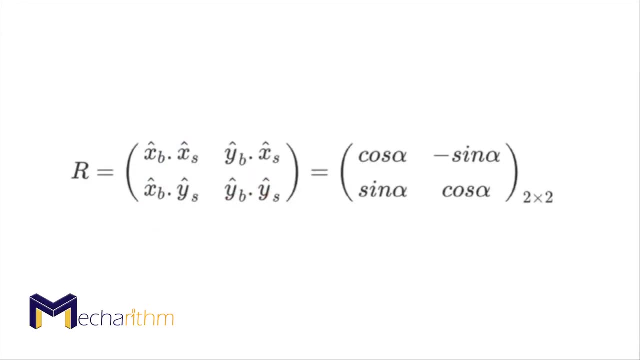 can be expressed as the projection of one vector onto the other multiplied by the lengths of the other vector. The two-by-two rotation matrix belongs to the four-dimensional space, subject to the three constraints. These constraints are: each column of the rotation matrix is a unit vector. 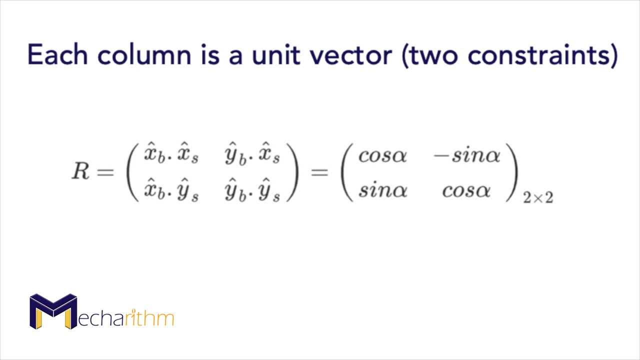 In other words, the rectangle of the B-frame is the unit vector. the lengths of the column vectors are one, and this is obvious because the column vectors of the rotation matrix are coordinate frames And also because these coordinate frames are orthogonal to each other, then the dot product of the columns is zero. Thus we have one degree of freedom. 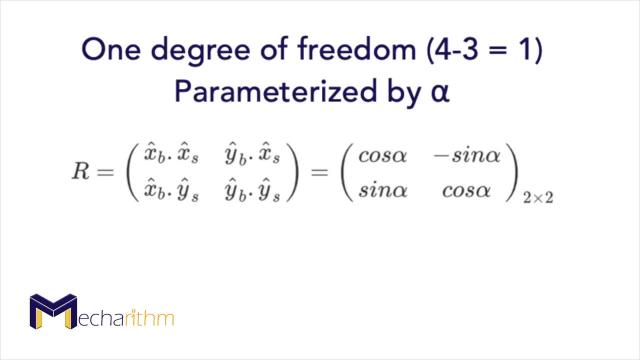 which is parameterized by the angle alpha, to represent the orientation. So recall that for d space minus three constraints, we would have only one degree of freedom, which is alpha, and this alpha can represent the orientation. The rotation matrix is an implicit way to represent the orientation, since we used 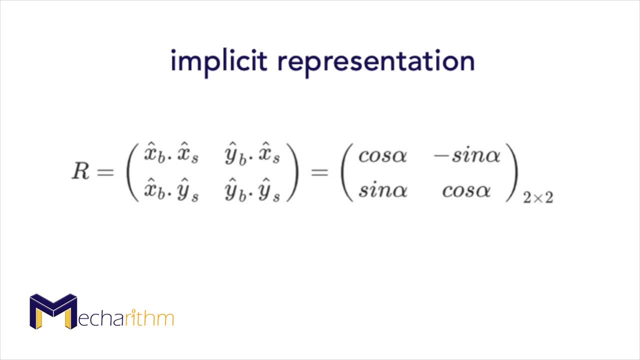 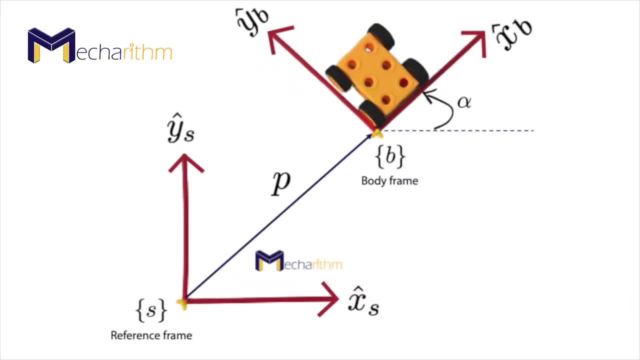 four parameters subject to three constraints, to parameterize alpha. Now that we found the way to represent the orientation of the toy car on the plane, it's time to represent this position. The position of the origin of the body frame and base frame coordinates can be expressed as the vector P from the origin of the S. 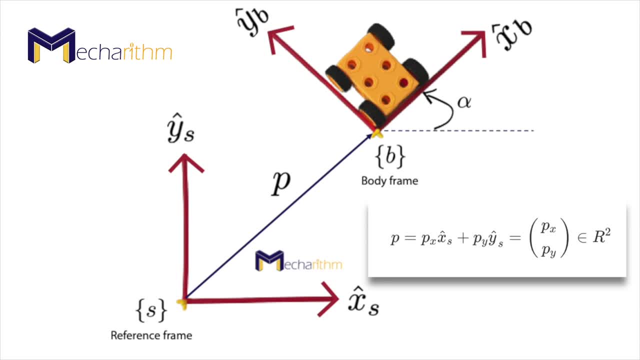 frame to the origin of the B frame. Thus, the configuration of the toy car can be represented by the pair R and P, which is the description of the orientation and position of the B frame with respect to the S frame. This means that base frame S. 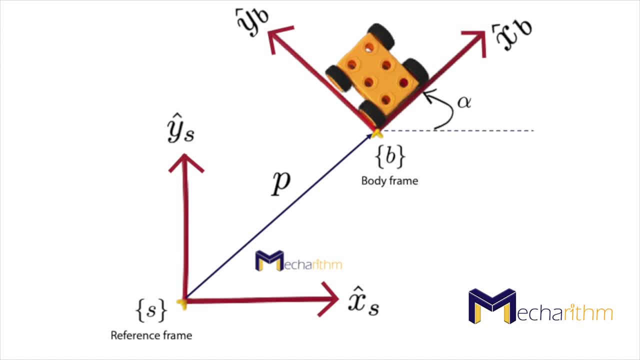 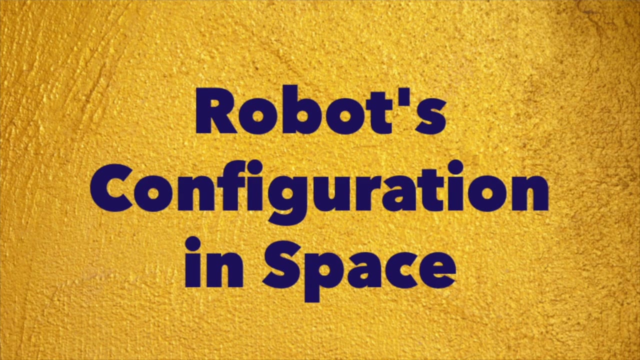 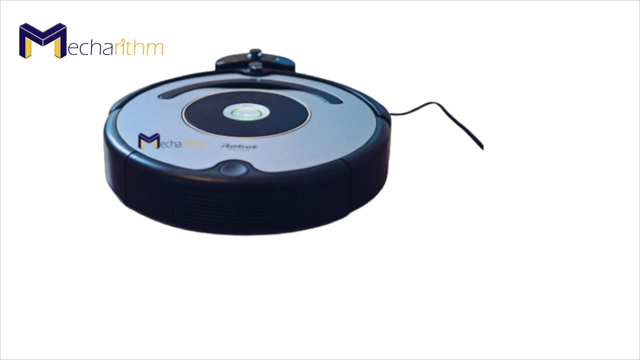 can be coincident with the body frame B by rotating the base frame coordinates around the S frame, the Z axis by alpha and then translating the origin by P. Using a similar approach, we can express the configuration of a robot in a space. We can use frames to do this, One simple way to represent the position and 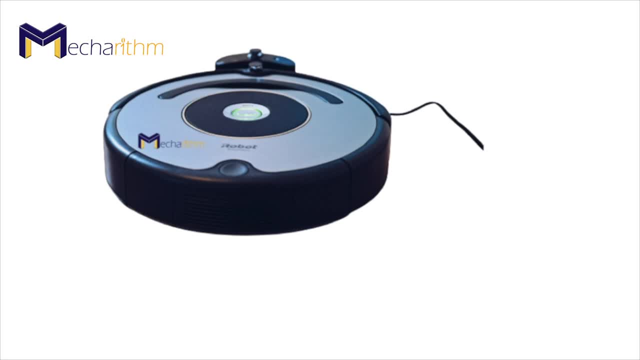 orientation and thus the configuration of a robot in a space, follows the best of these steps. We first fix a frame to the body of the robot according to the right-hand rule. Sometimes this frame is attached to an important point in the rigid body, like the center of mass, but this is not required. And then we fix a